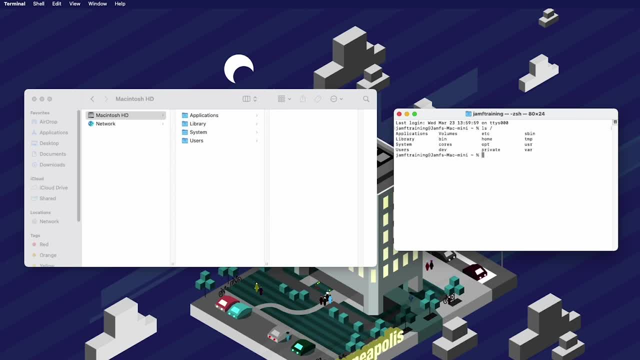 ls forward slash, where the forward slash indicates the root level of the disk. We see there are many more items visible in the command line compared to the Finder. This is because the Finder hides items that are of no use to the user. If they were visible, users may try to move or delete. 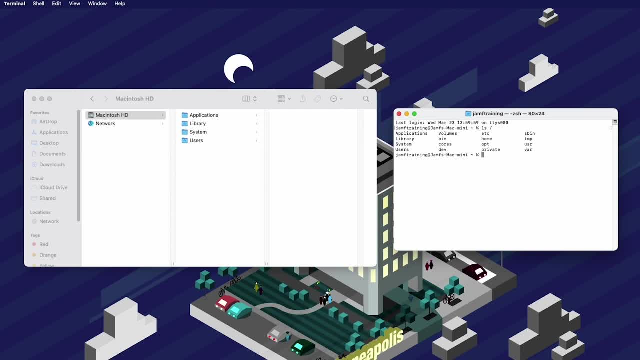 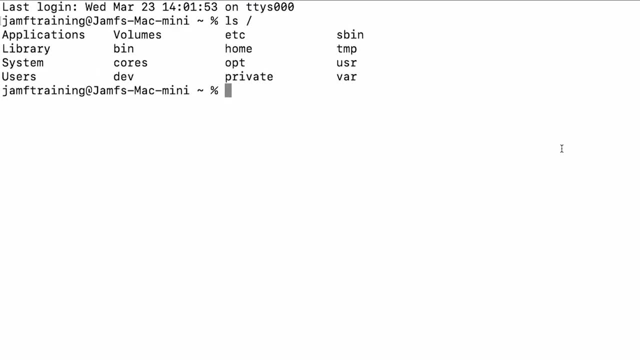 these files which could be detrimental to the functionality of the computer. I'm going to enter full screen in Terminal and make the font size bigger so we can focus on the command line. Let's look at the structure of a command. A command is a program that tells the computer 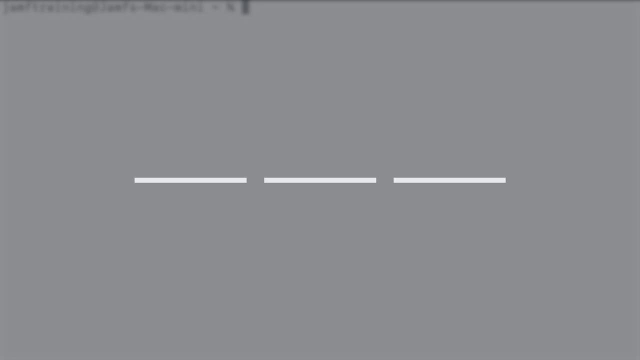 to perform a task and is made up of three parts. First, it contains the command itself, like the list directory contents command we've been using. Second are options for the command. An option can change the way a command is performed and is preceded by a hyphen. 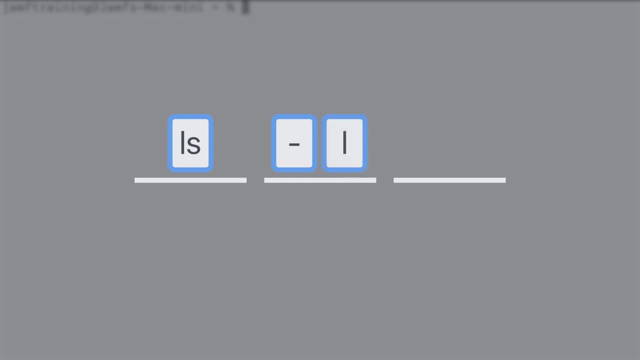 So if we add a space after ls followed by hyphen l, this will list items in long format, which expands the information returned. The third part is an argument. An argument indicates what the command should perform its actions on. So far, we've been using a forward slash to indicate the root directory, So putting 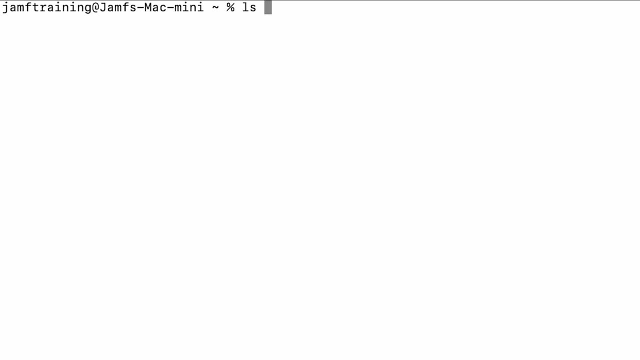 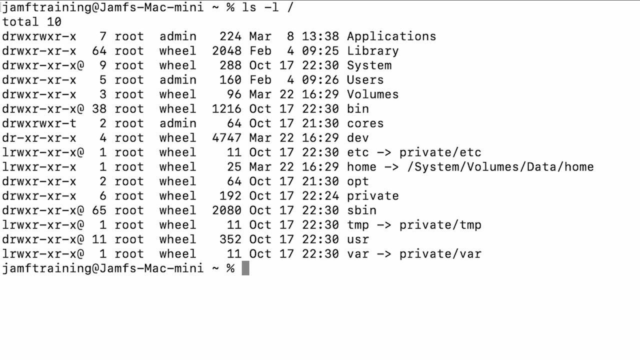 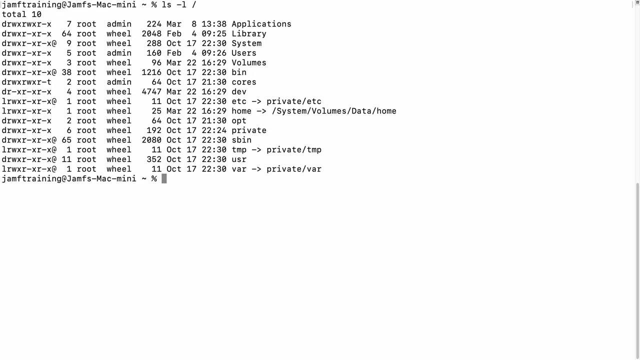 this command all together by typing ls hyphen, l forward slash results in a list of all items in the root directory in long format. For most commands, more than one option can be strung to each other. Let's type the same command, but this time include a capital T after the l option. 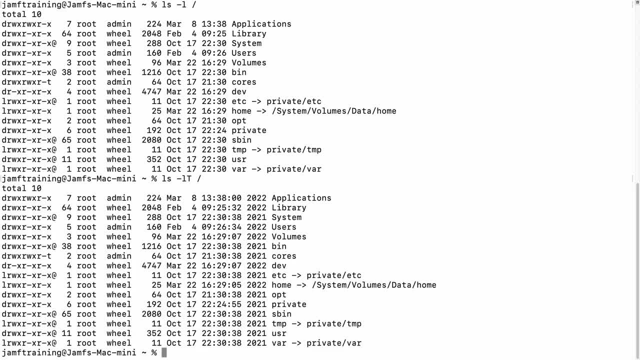 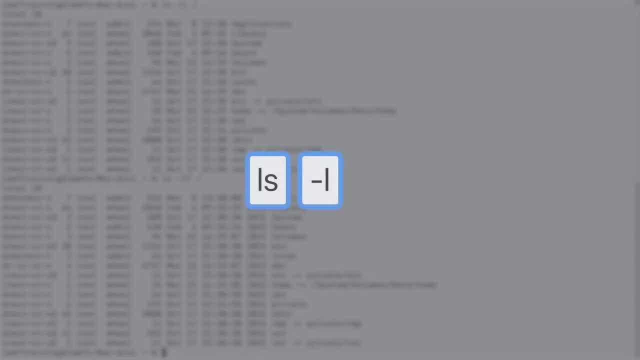 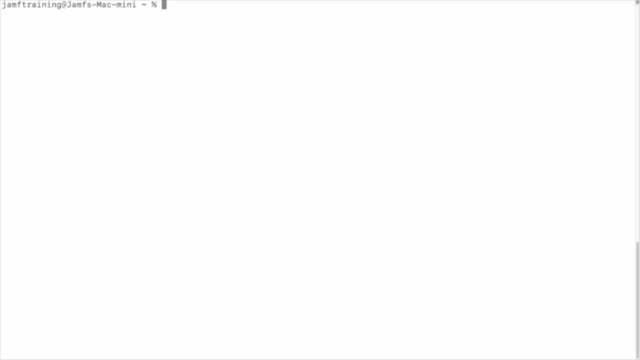 When used with the lowercase l option, this displays the complete time information for each item, now including seconds and years. It's important to note commands, options and arguments are all case sensitive. Upper and lowercase characters can have very different meanings. To know what available options there are for a specific command, we can review the 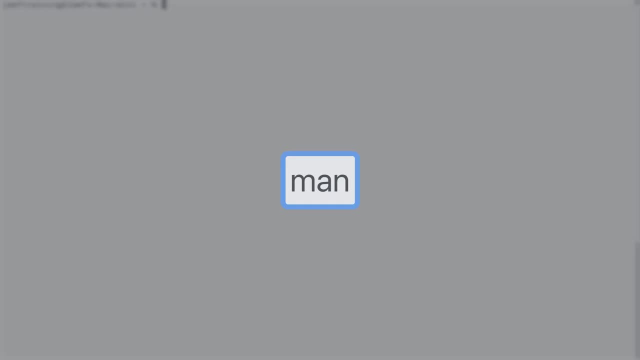 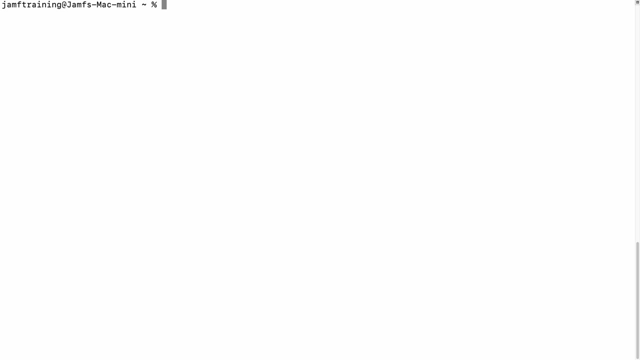 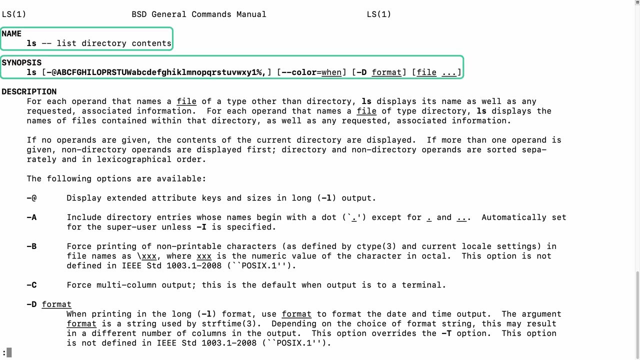 command's manual. To access manual pages, type man, followed by the name of the command. to look up, Let's use the same list directory contents command and access its manual page by typing man, space, ls. Here we see the name of the command, followed by a synopsis and description.